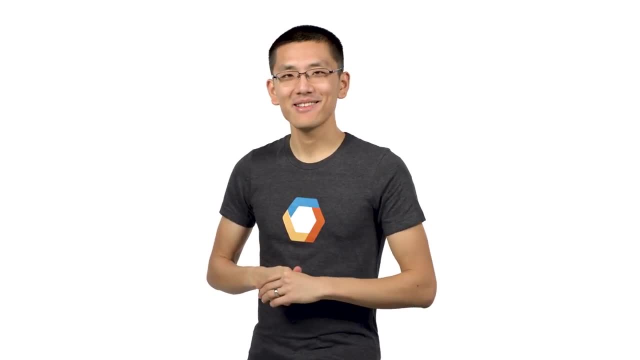 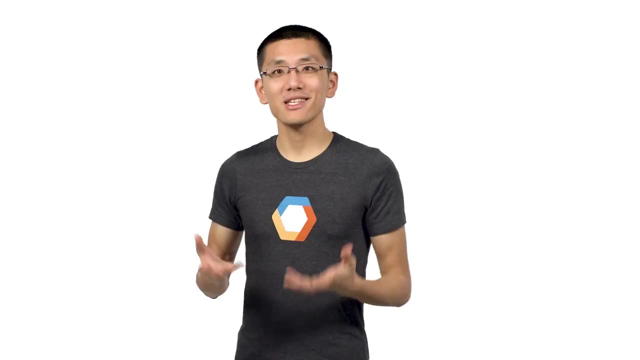 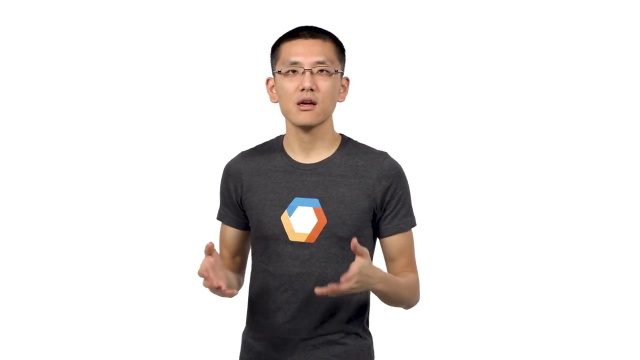 The only thing better than data is big data, But getting your hands on large datasets is no easy feat. From unwieldy storage options to difficulty getting analytics tools to run over your dataset properly, large datasets can lead to all sorts of struggles when it comes to actually doing. 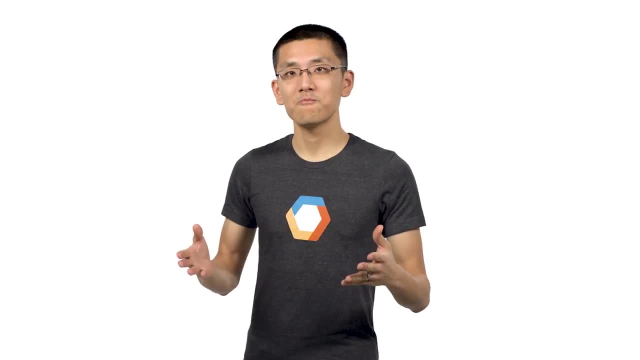 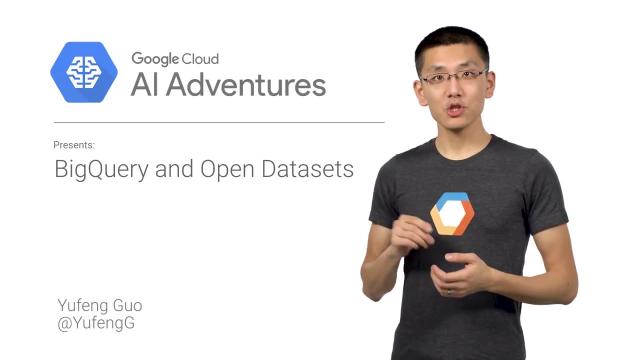 something useful with them. So what's a data scientist to do? Stay tuned to find out. Welcome to AI Adventures, where we explore the art, science and tools of machine learning. My name is Yufeng Guo, and on this episode we're going to check out the BigQuery public. 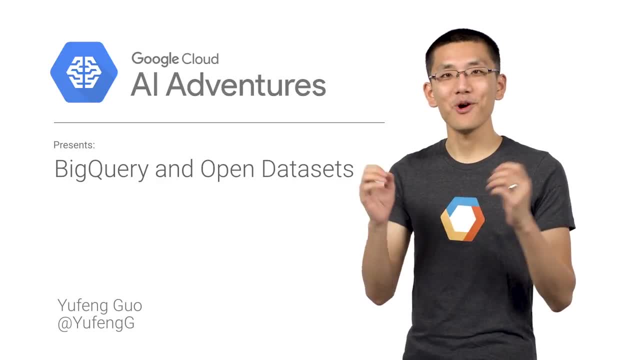 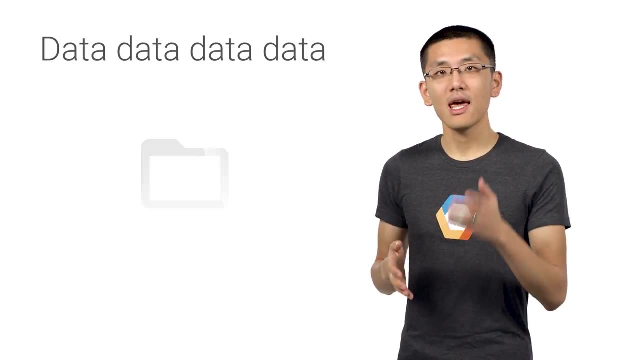 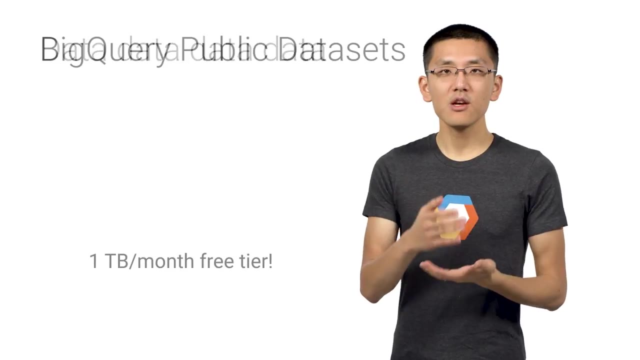 datasets and explore the amazing world of open data. We all love data, preferably the more the merrier, But as file sizes grow and complexity increases, it becomes increasingly challenging to make practical use of that data. BigQuery public datasets are important to us because they can give us a wonderful Online data cycle. 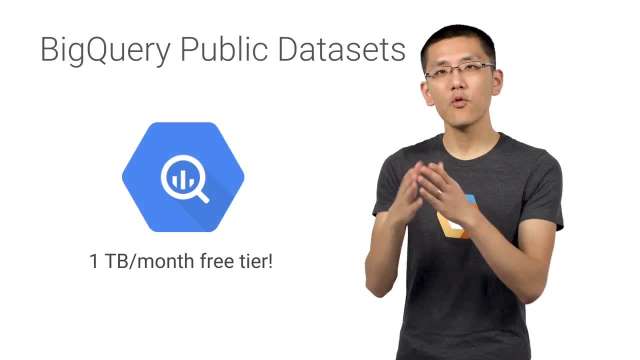 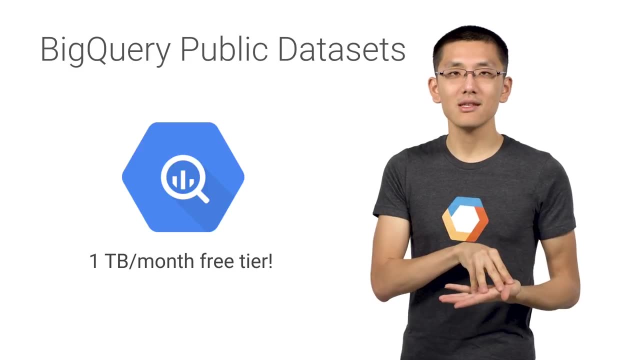 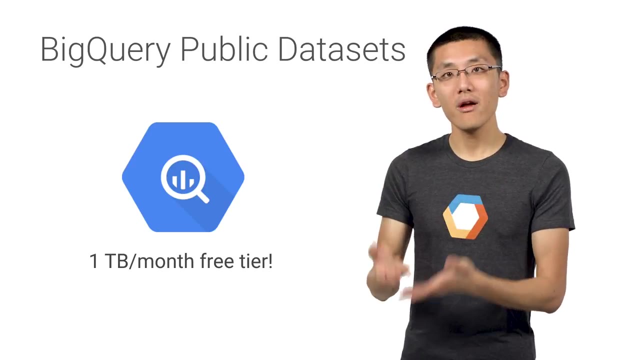 public data sets are data sets that Google BigQuery hosts for you to access and integrate into your applications. So this means that Google pays for the storage of these data sets and provides public access to the data via your cloud project. You pay only for the queries that you perform on the data. 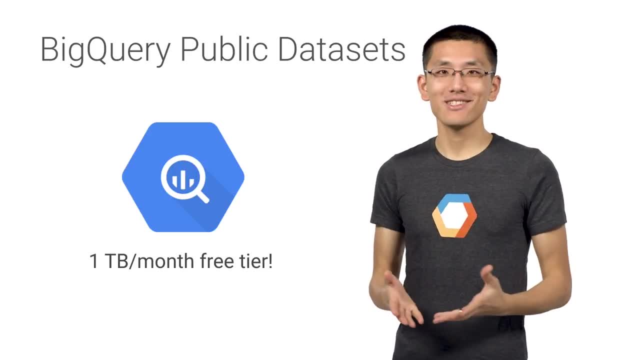 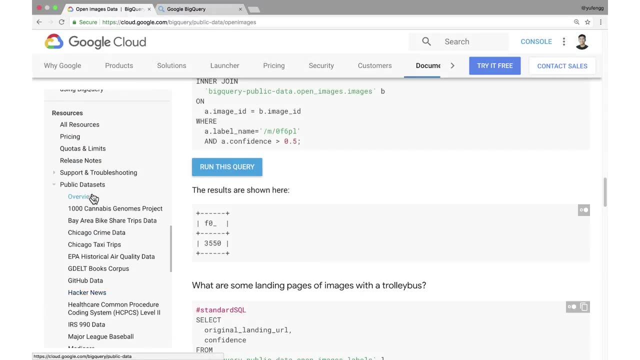 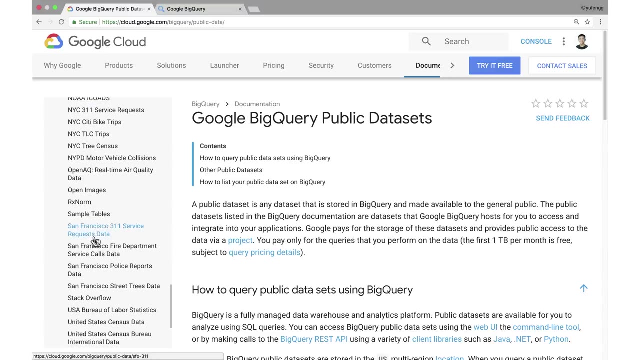 Moreover, there's a one terabyte per month free tier, making getting started super easy. Looking at the public data sets page, we can see that at the time of this recording, there are nearly 40 public data sets. Each data set in turn has many tables. 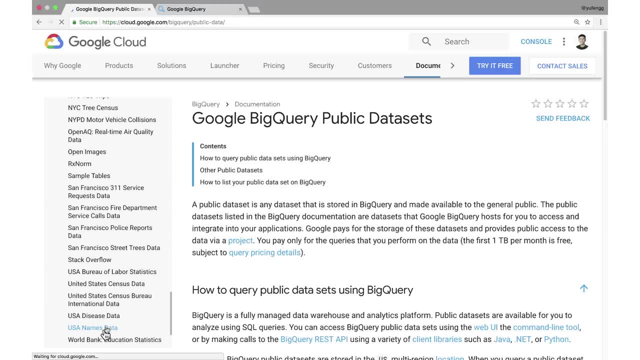 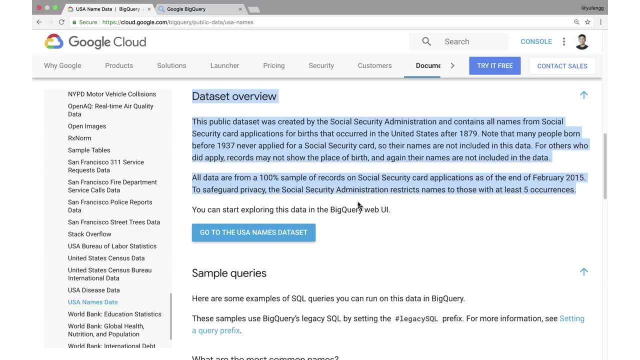 Thousands of queries from hundreds of projects all over the world are already making use of these vast public data sets. What's really neat, though, is that each of these data sets comes with a bit of explanatory text that helps you get started with querying the data. 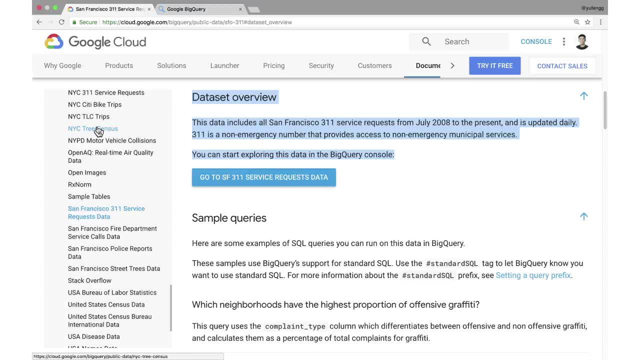 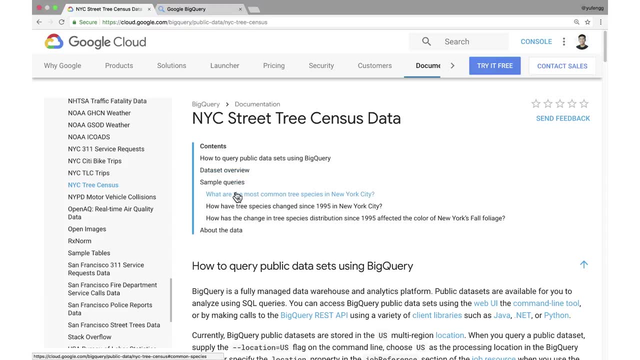 and understanding its structure. Let's take a look at it. For example, here's the New York City Tree Census. The page shows us how we can easily find answers to questions like: what are the most common tree species in New York City? 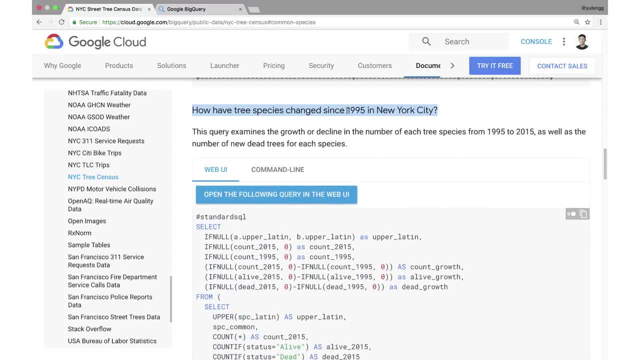 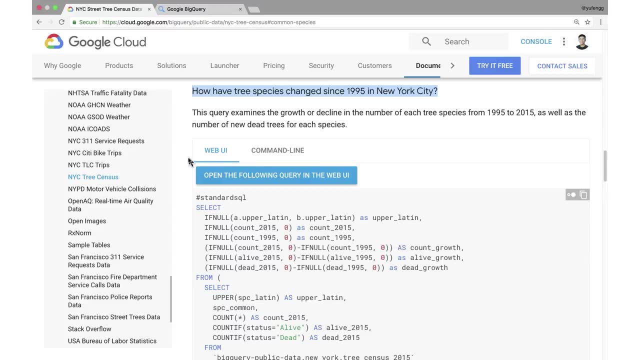 And how have the tree species changed since 1995 in New York City. These are all accessible by literally one click from the Docs page, which opens right into the BigQuery interface. Another data set that is quite amazing is the Open Images data set.